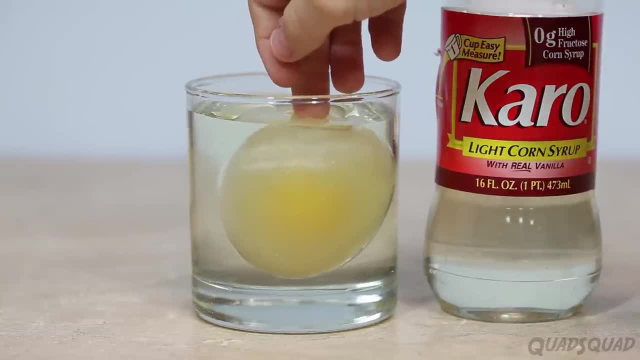 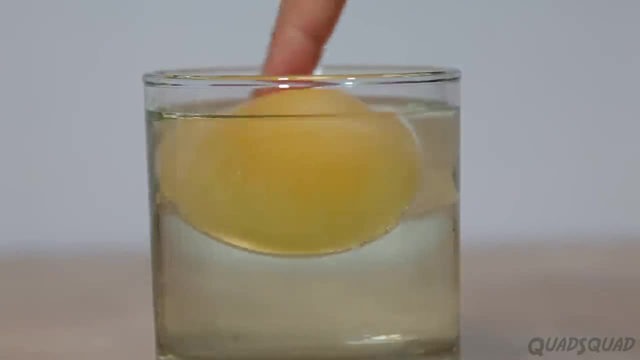 We want all of it underneath. You'll notice after a few hours there will be this liquid on top and you're going to want to pour that out because otherwise it will be sitting in the vinegar. Pour off the top vinegar and 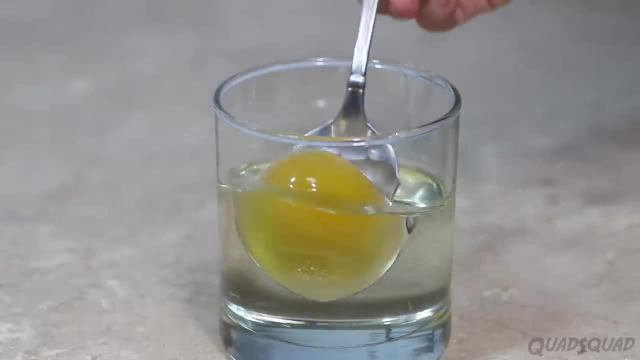 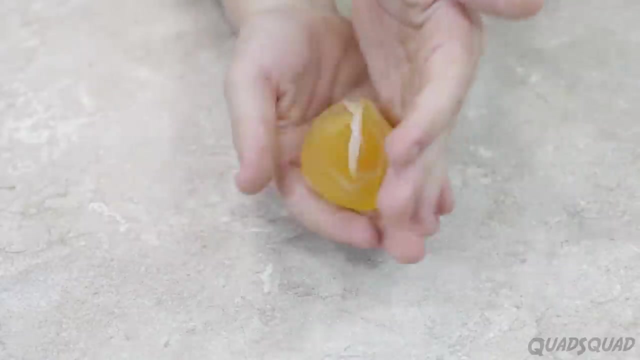 put your egg back in there again And leave it overnight. This is what it looks like once most of the liquid has been removed. As you can see, really all of the vinegar is out And a lot of the liquid from the egg is out. 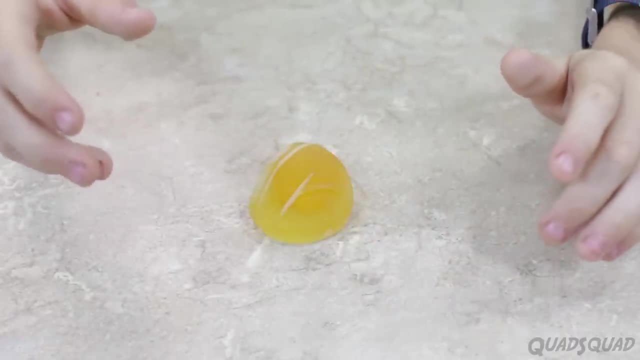 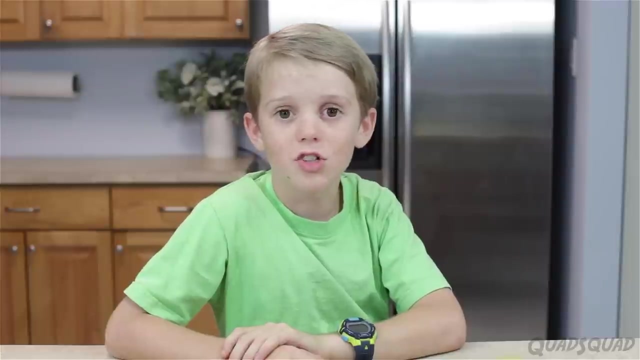 It's definitely not bouncy anymore. So we took the shell off, which also added liquid in the egg. Then we took the liquid out of the egg. Now we're going to show how to get the liquid back in the egg. 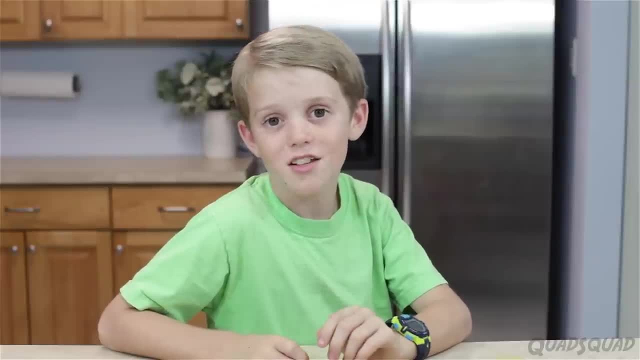 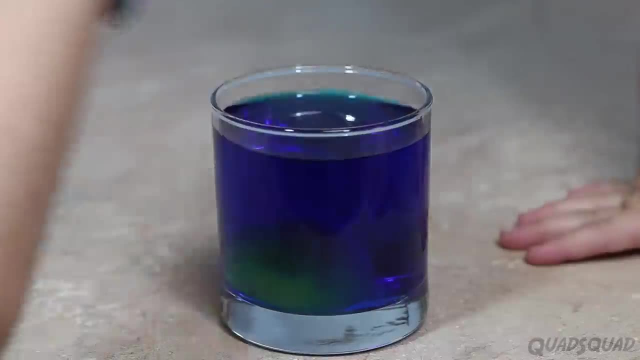 Remember this is not magic. Remember this is science. Take a cup of water, add food coloring which you want your egg to look like and gently add your egg, Leave it for a few hours and then pull it out and it should look something like this: 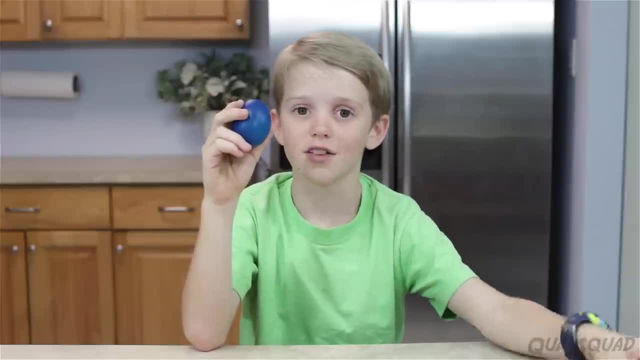 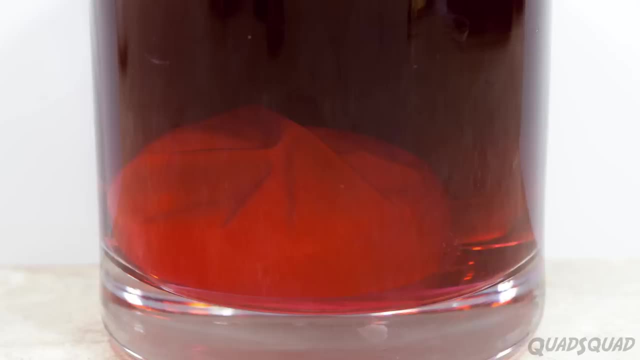 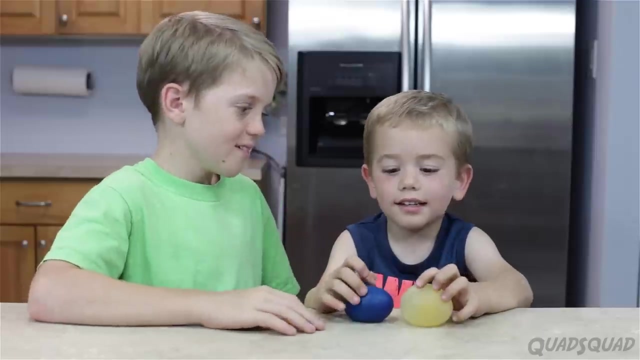 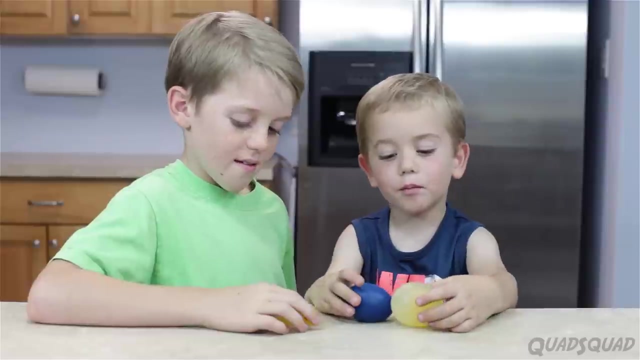 Now, this is actually the same size as this, but with color which is even cooler. Want to see it up close. Now I get it. It's not magic, It's science. Yup, It's osmosis. I wonder if we could, when we could, open it and these eggs would explode everywhere. 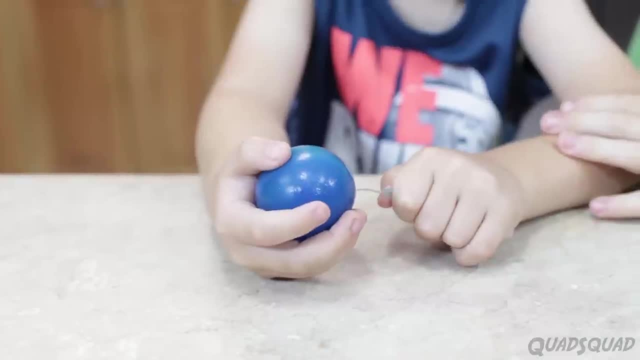 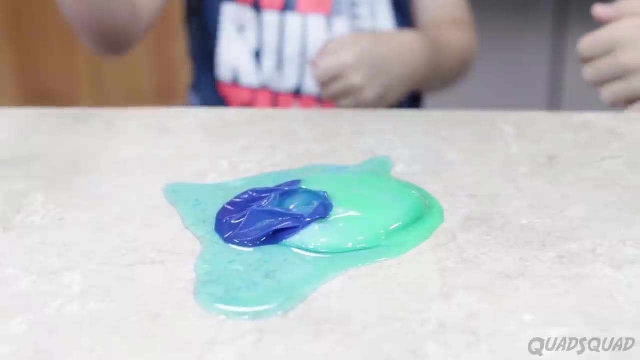 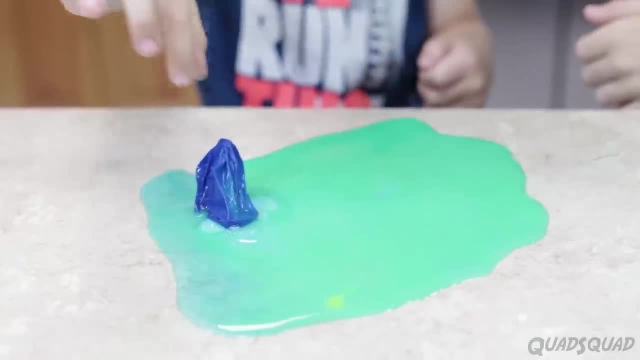 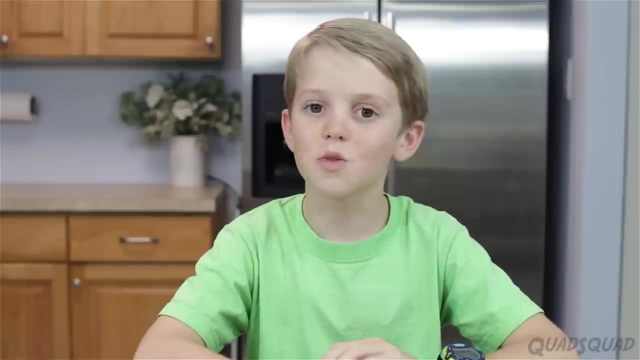 It's amazing, Amazing, It's amazing, It's amazing. Through osmosis, we're able to add and remove liquid from our egg. This was a really fun experiment. I hope you learned as much as I learned. Don't forget to subscribe. 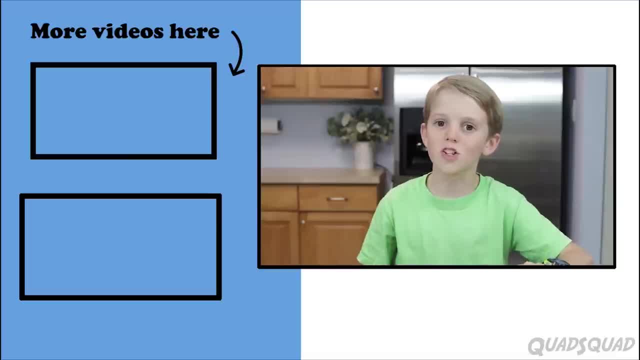 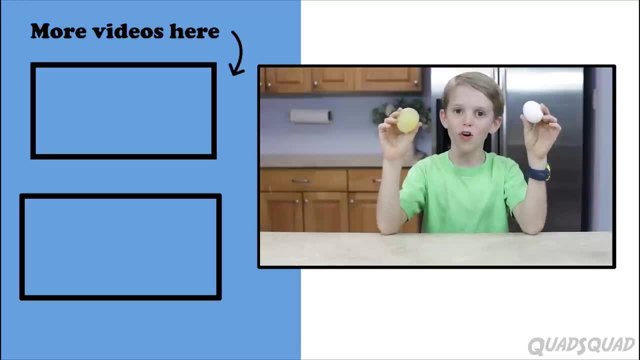 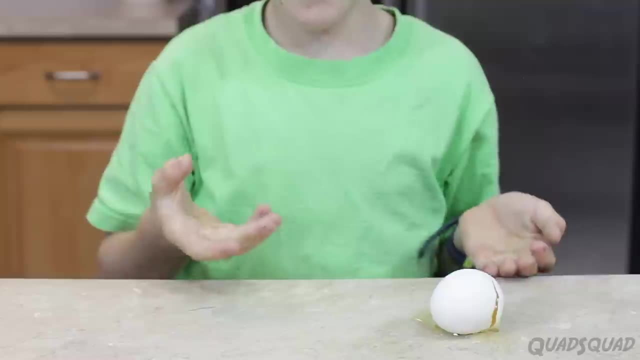 If you haven't seen our other videos, click here. Thanks for watching my video. Bye, Two eggs: one with a shell, one without a shell. Who will break and who won't? Let me know in the comments. Bye. Bye.